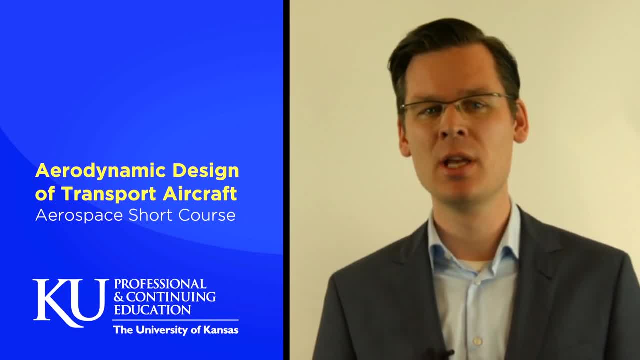 Transonic flow characteristics and their effect on aerodynamic performance is therefore an important aspect of the course. I will explain how these effects limit the 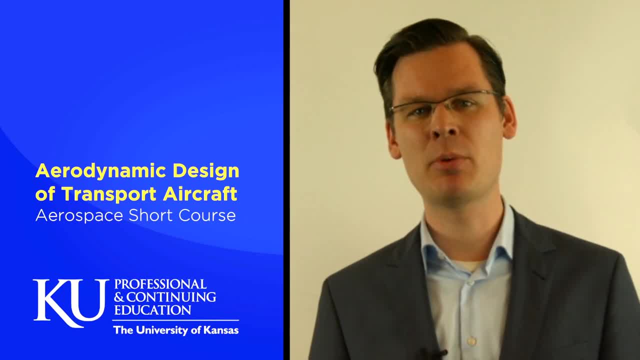 aircraft performance in terms of speed and lifting capability at high Mach numbers and what design measures can be taken to mitigate these effects. 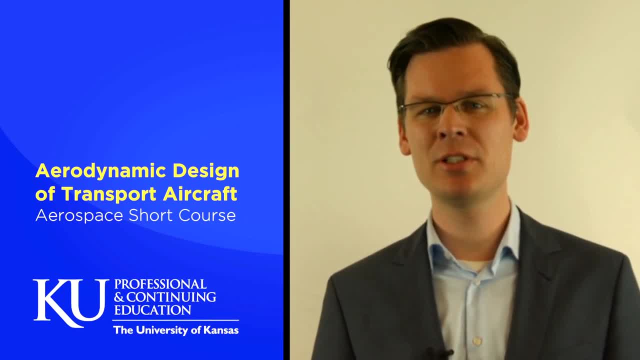 But did you know that transonic effects can also limit the lifting capability at low Mach numbers, for example at landing speeds? Flow over wing leading edges or slats can accelerate to supersonic speeds effectively limiting the lifting capacity of the wing. I will present 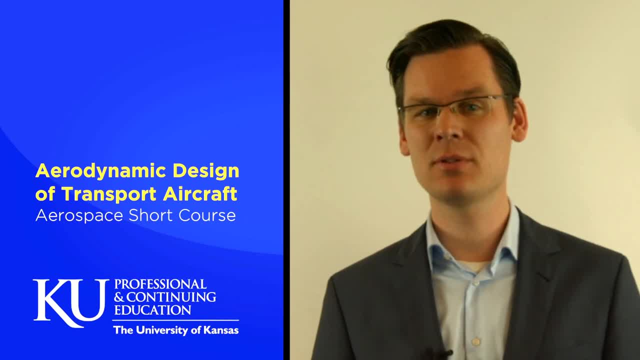 good practices for the design of high-lift devices such as flaps and slats. 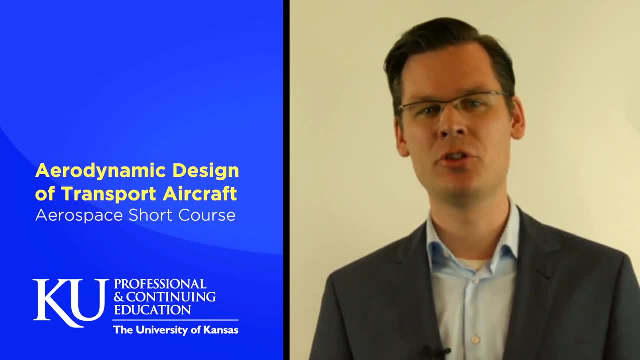 The aerodynamic design of the aircraft determines the aerodynamic performance of the aircraft at low and high speeds. At high speeds I will show how the aerodynamic performance changes when the Mach number gets close to one. I will explain the causes for drag creep and 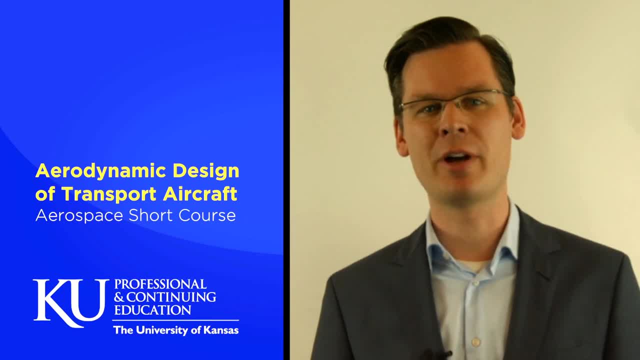 drag divergence and in addition I will present the mechanics of high-speed buffeting and the effect on the caving of transport aircraft. 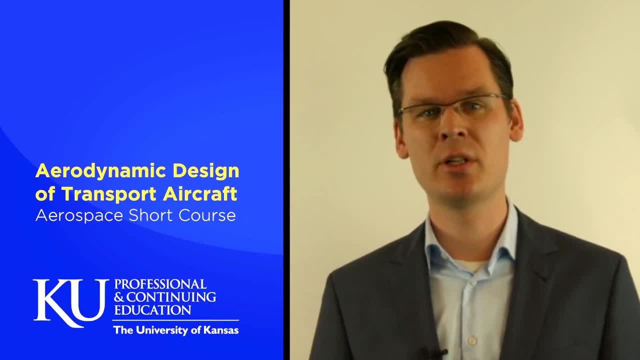 We will also investigate how the stability and control properties change when an aircraft towards the dive Mach number. 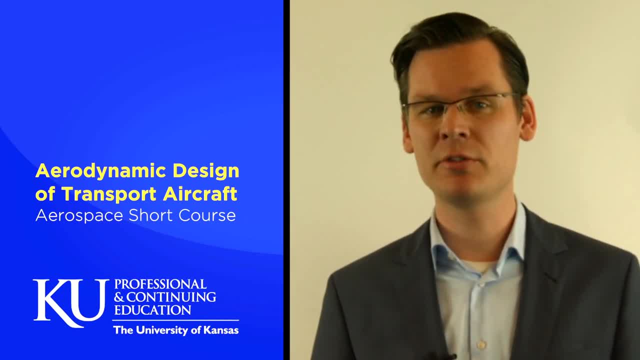 I will show why virtually all modern transport aircraft and business aircraft that cruise at high Mach numbers require an all-moving tailplane. Finally, I will demonstrate how wing design parameters influence the aerodynamic and flight performance at these high Mach numbers. 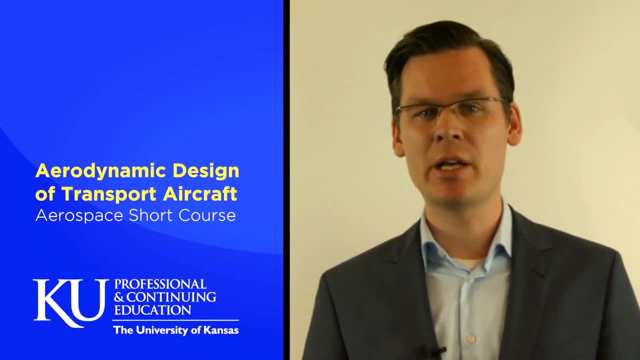 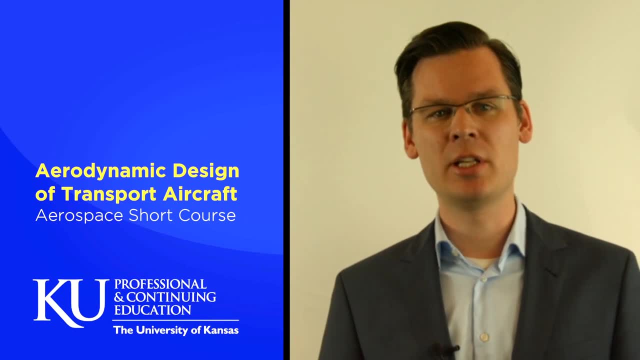 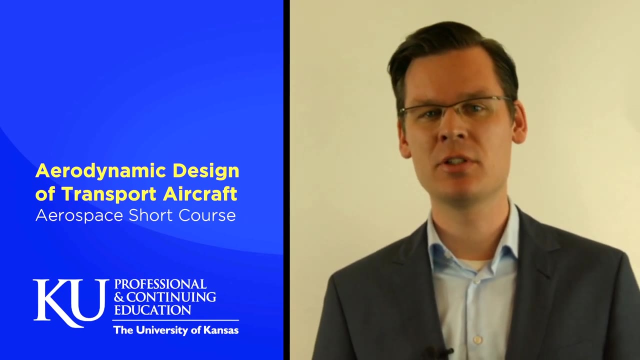 In addition to the state-of-the-art in aerodynamic design, I also discussed the impact of new technologies on the aerodynamic performance of the aircraft. This includes the aeroelastic effects of flexible composite wings on the aerodynamic efficiency of the wing and the control effectiveness of ailerons. 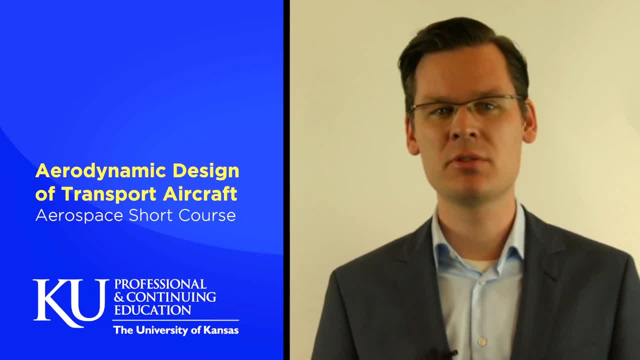 Additionally, we will investigate the challenging contradictions that exist in designing a swept wing with extensive laminar flow. 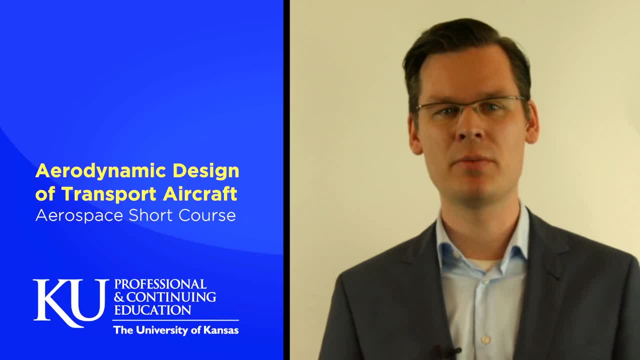 Finally, we look at the integration challenges that arise from the introduction of progressively larger turbofan engines.